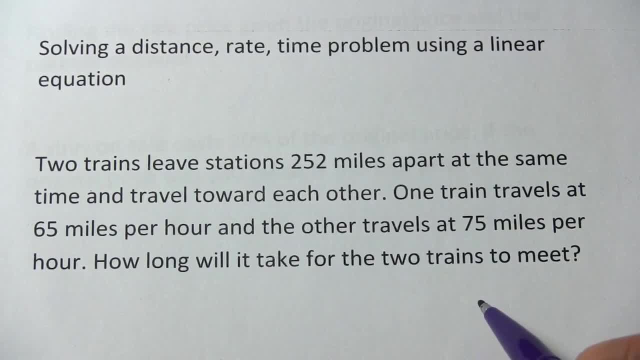 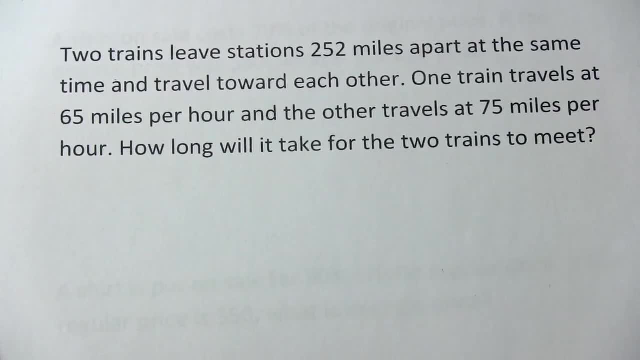 per hour, and the question is: how long will it take for the two trains to meet? So this might seem like a really difficult problem. I think the best way, when you're dealing with distance, rate and time and you've got two different objects, two different trains, is to make a chart. 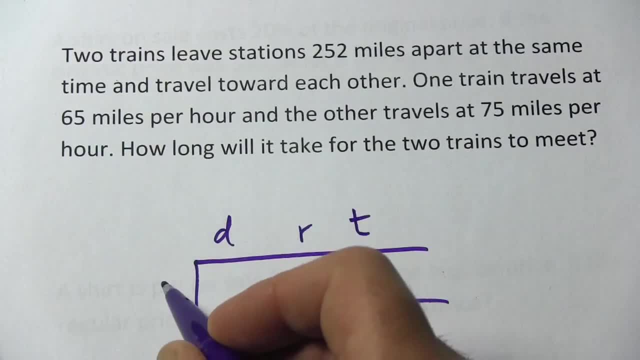 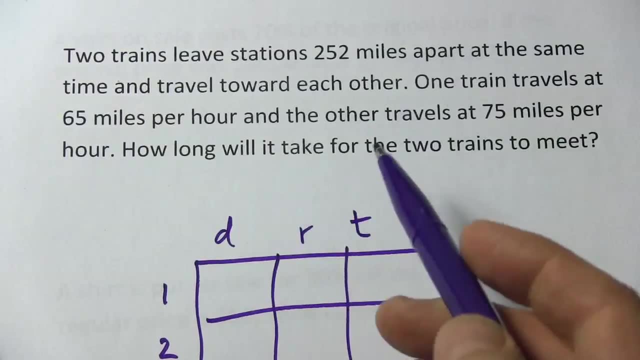 and fill in whatever you can. So we're going to call this train one and this train two. So I'm going to start with what we know, what jumps out at me. Let's see, train one is going 65 miles per hour, so I can fill that in. Train two is going 75.. 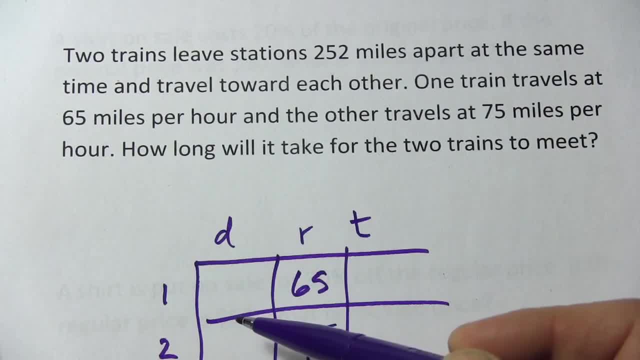 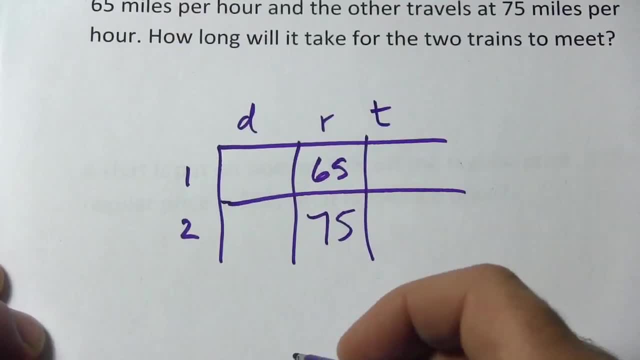 The total distance is 252, but I don't know how far they're going to. each of them is going to travel during that time. I'm going to come back to that. Let's think about the time for a minute. If you've got two trains and one leaves over here, 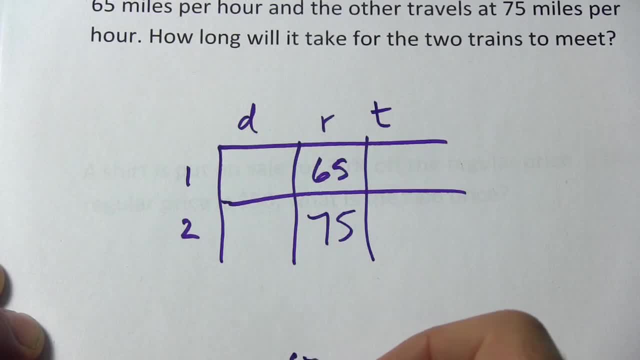 and one leaves over here at the same time. they're going to meet somewhere in the middle. they're going to meet at the same moment. So since they left at the same time and they meet at the same time, they both travel the same amount of time. 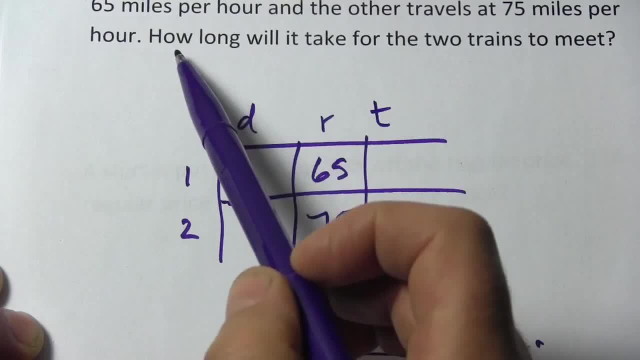 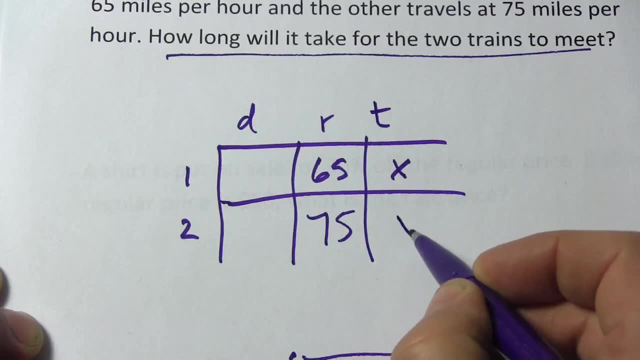 What varies is the distance. So- and this is actually what we're looking for- how long will it take the two trains to meet? So we're going to call that x and it's going to be the same for both of them. So I can, I can fill that in with a. 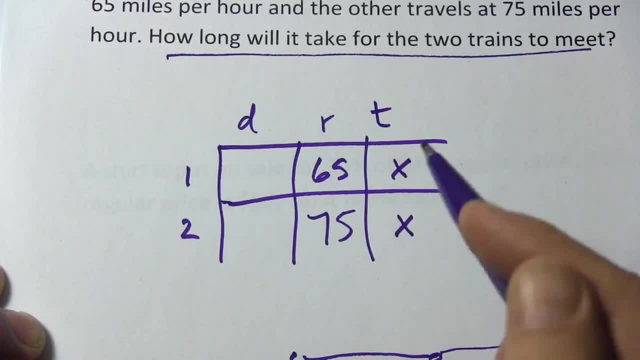 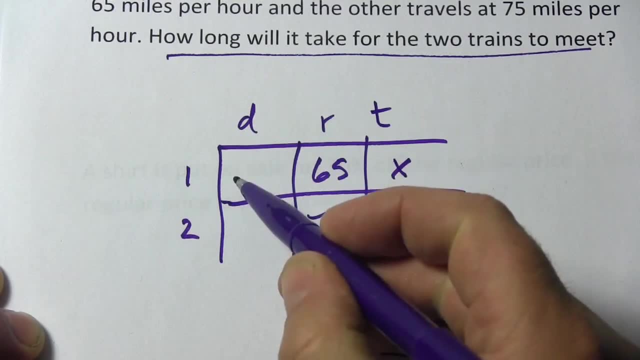 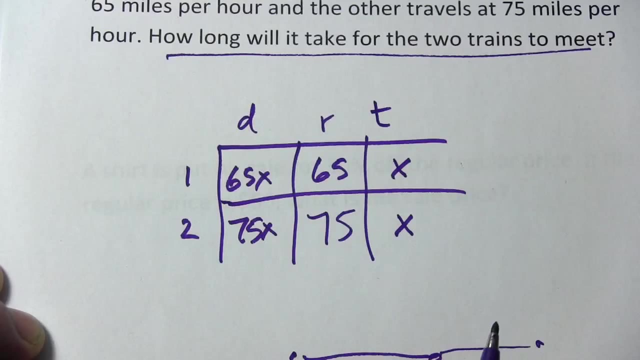 variable. Now let's think about the distance. Distance equals rate, times, time. So the distance train one travels is just 65x, And the distance train two travels is going to be 75x. Now I've got one other piece of information up here, and that is: 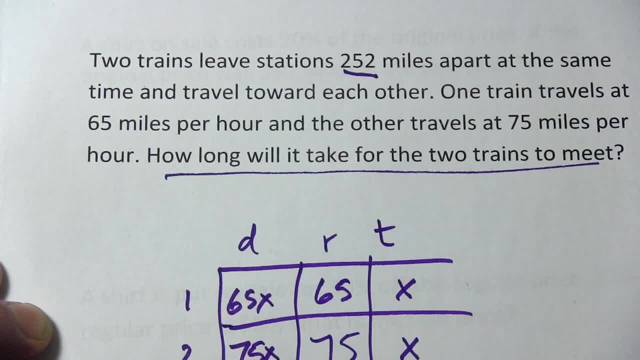 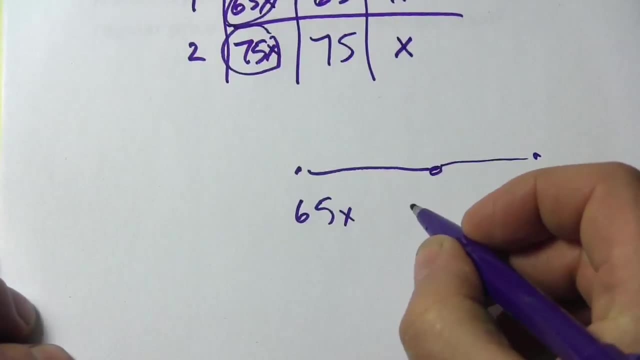 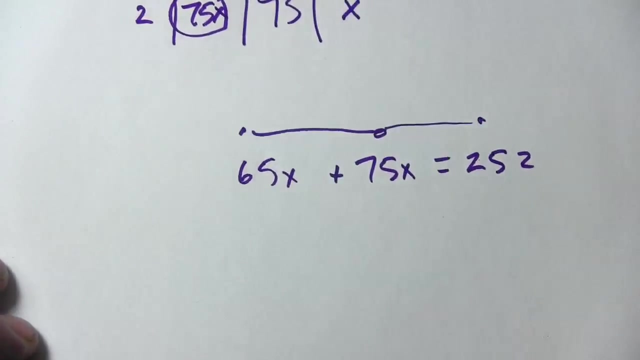 the total distance. They're 252 miles away, Which means that this distance that train one travels plus this distance that train two travels is going to add up to 252.. And that's the key to solving this. I can simply write: 65x plus 75x equals 252.. What I've got now is an equation with one.